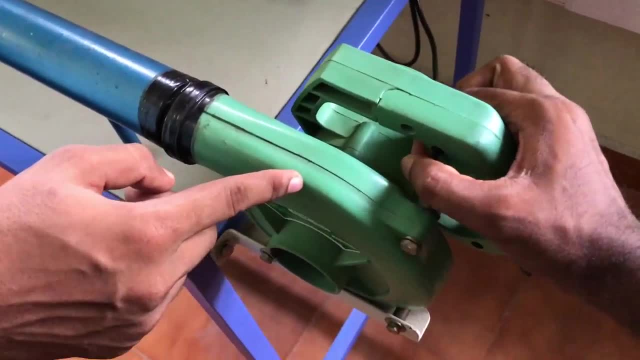 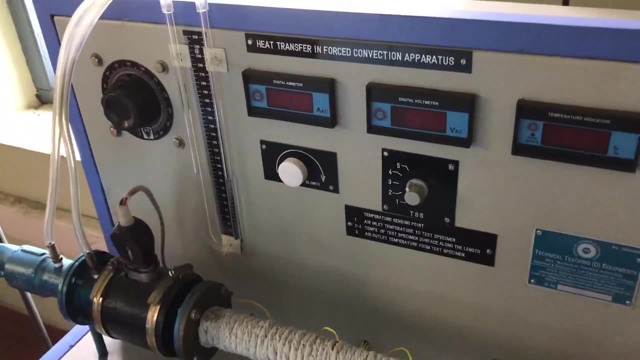 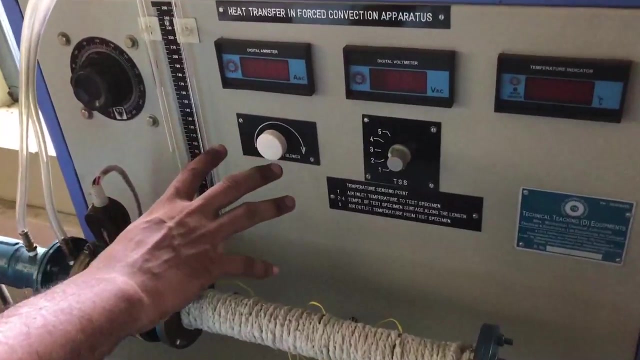 to permanently keep it in the on state. So blower is on Now. this is the dimmer for this one blower. That means now blower is on. and by adjusting now first, initially this should be kept at the zero position, And after that we will be adjusting it And 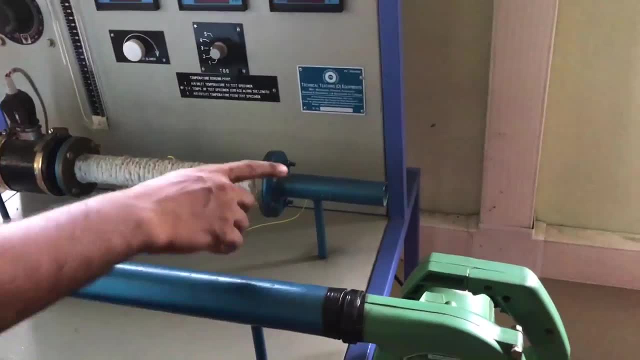 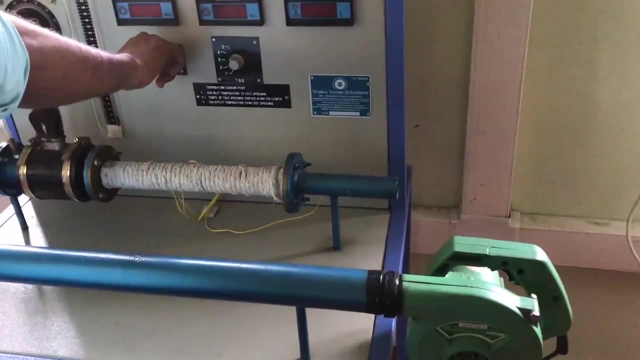 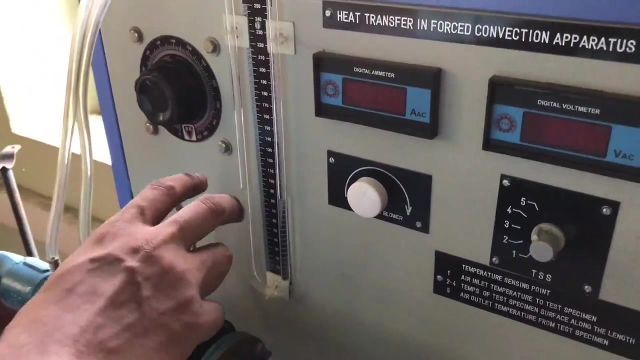 after adjusting it, this blower will start working And the air will be flown out of now. Now we can regulate the flow from the blower. So as we increase this flow, what happens is there will be a level difference in this U2.. And because of that level difference, 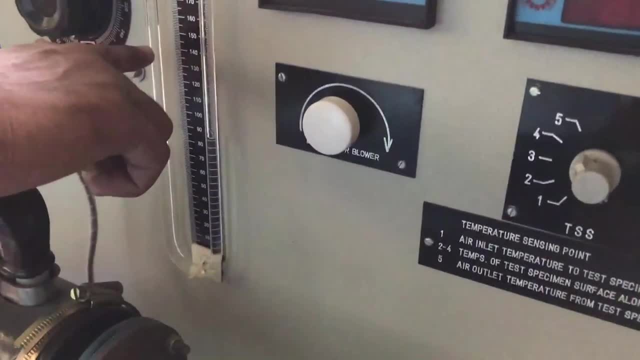 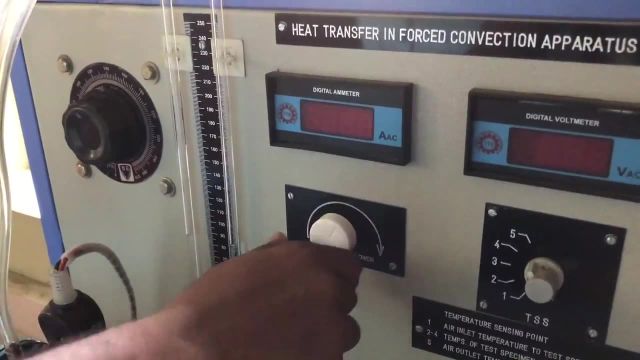 we are able to note the level difference. So let us say that here the reading is H1 and here the reading is H2.. So we should set this blower, this dimmer, at a position so that we are able to control the flow at a given level difference. It will be given. 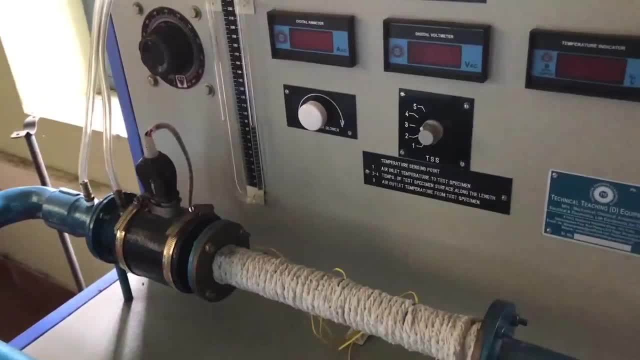 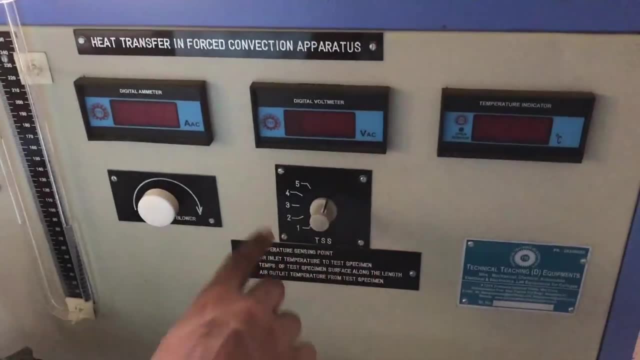 in the question. The flow will be at this, At this much height level difference. So we should keep that. Then, after that, what we do is, initially we will be taking this T1, T2, T3, T4 and T5. And then after every, 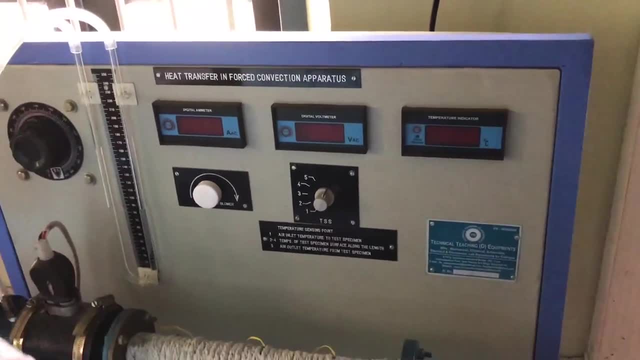 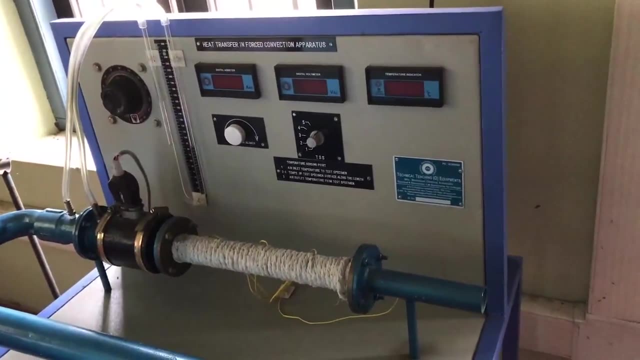 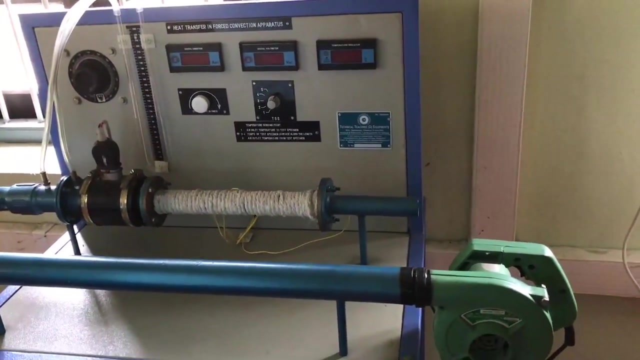 turn intervals. we will keep on taking reading And at a time this T1 to T5 reading will be same as that of the previous set And at that state we can say that our entire attack is in steady condition And now we have readings. So now take the average. 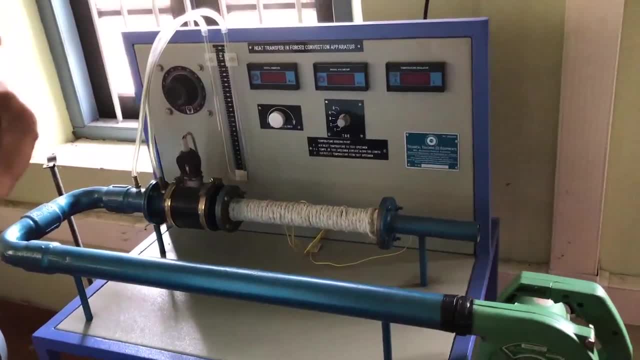 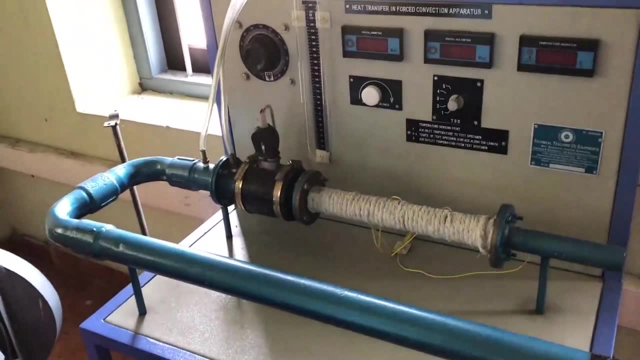 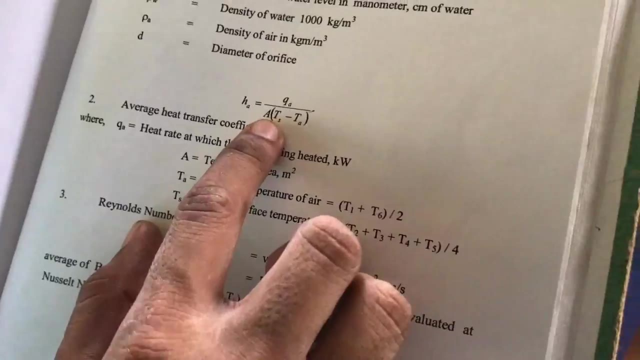 of T1 and T5. So we are able to get the temperature of this area, Then T2, T3 plus T4 by 3, we will get the surface temperature, And here this heat transfer coefficient is QA by A into TS minus TA. So TS, surface temperature and TA are obtained. A is the 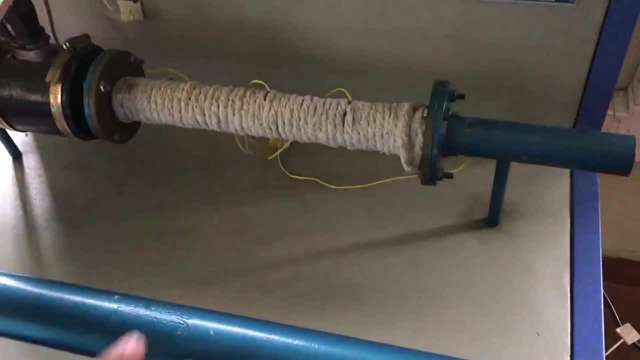 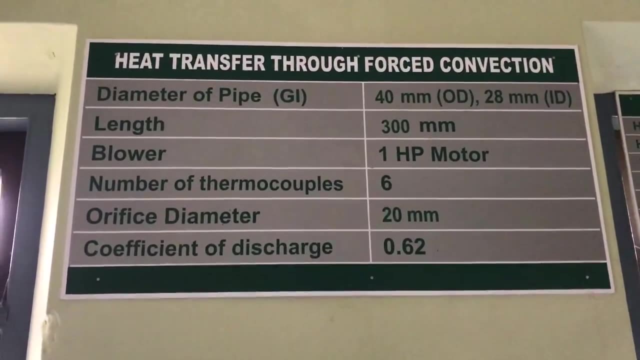 surface area, That is, the curved surface area of this one, this particular section, And that can be obtained by. here, diameter of the pipe and the length of pipe are given. So we are able, by PIDL, we are able to obtain the curved surface area. Now then, 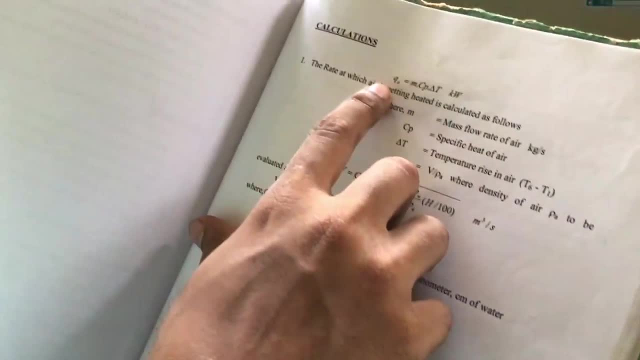 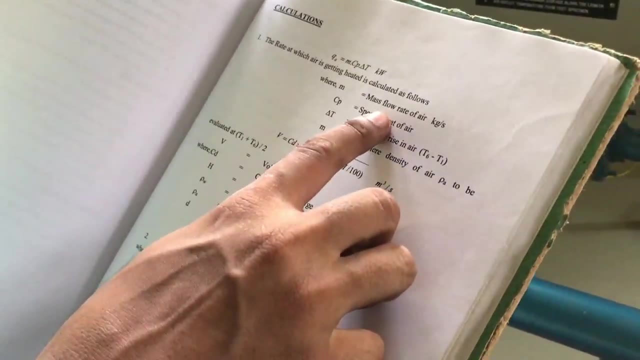 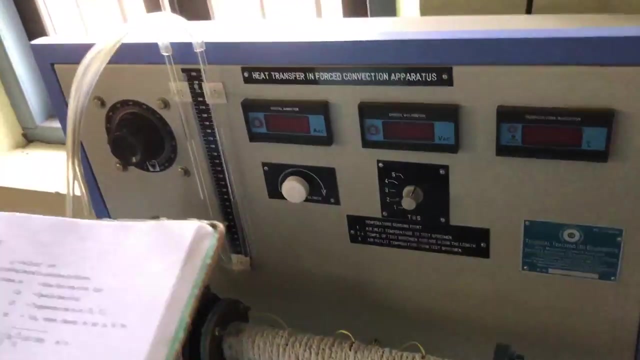 QA. QA means it is the heat supplied, That is, QA is equal to MCP into delta T, where M is the mass flow rate of the air. So mass flow rate of the air. for finding the mass flow rate, we are having the here. we are having the height difference, the level difference. 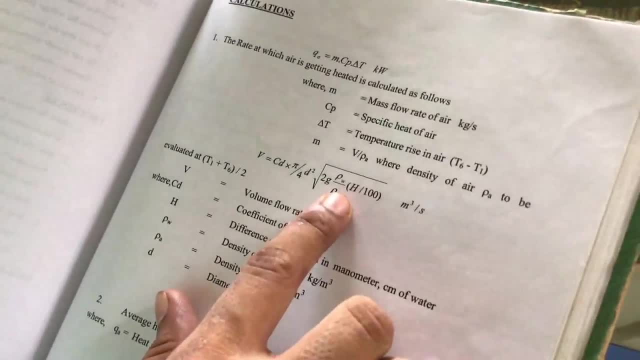 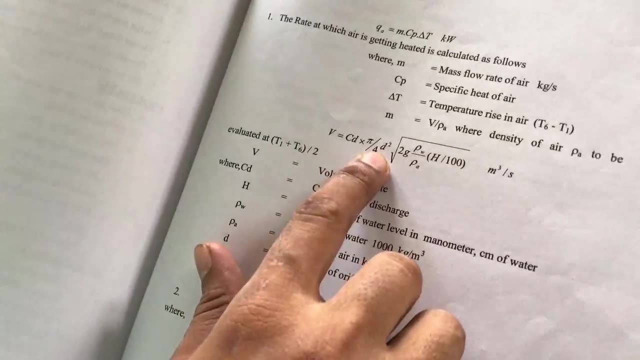 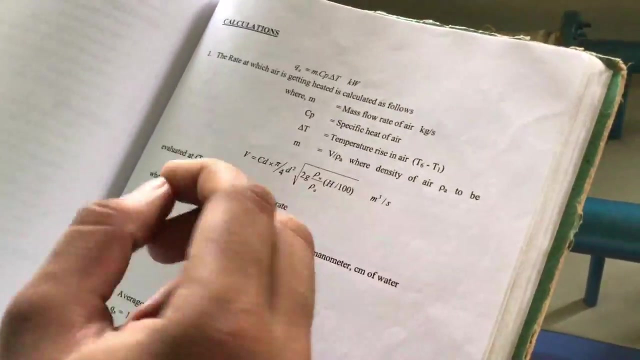 That is H And that H is substituted in this equation. Here we are having CED, That is this one coefficient of discharge. Then PI by 4 into D square. D square, there is a particular orifice meter. here There will be an orifice and the value of diameter of that orifice, 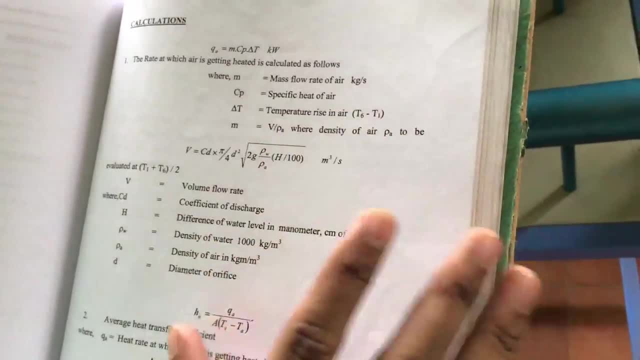 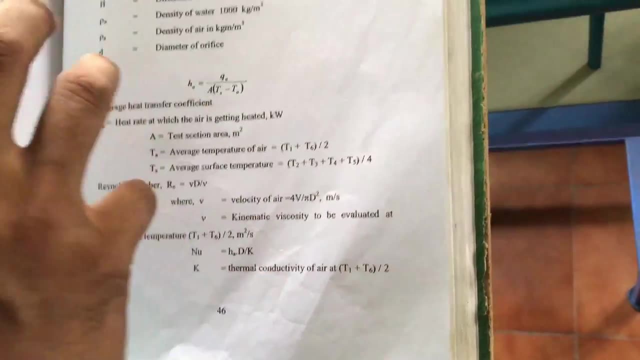 should be substituted here. So into 2G, into Rho, W by 2I, into H by 100, we will be getting the volume of discharge. Then that volume of discharge, when we are multiplying it with the density, we will be getting the mass flow rate. So into CP. CP is heat constant, constant. pressure And into T. So this is CED. So this is CED, This is CED, This is CED. So, from Q and the Qian, the total value of the water will be K, positioned down into delta. 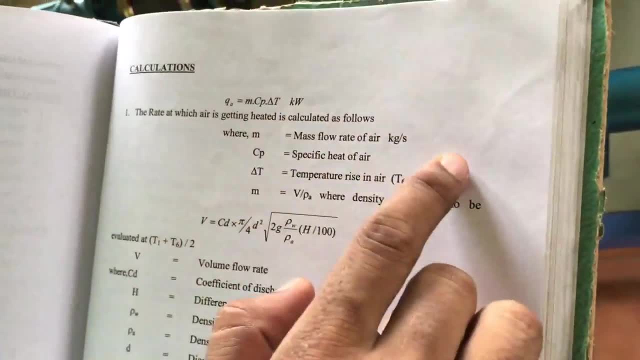 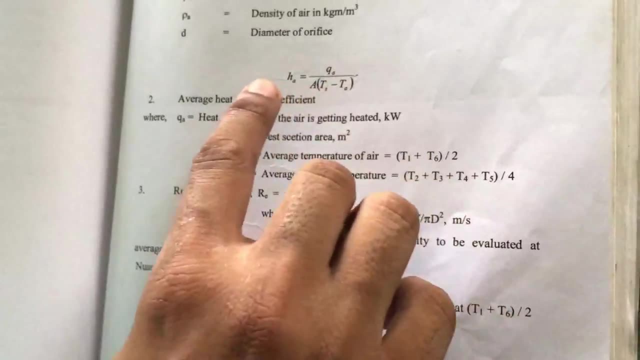 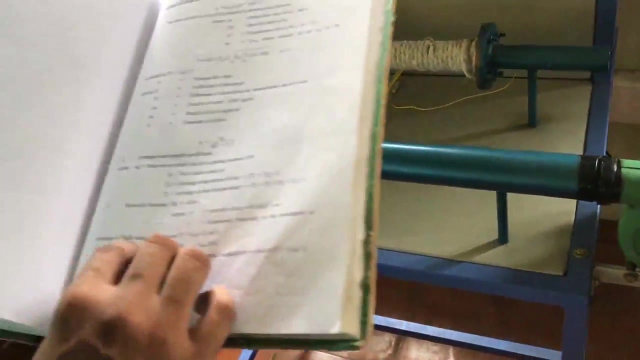 T, Specifically at constant pressure, into delta T. Delta T is TAS minus TA. We are able to get Q. So now by substituting the known values here we will be getting the commission in this forced convection. Similarly we can here we have T1 and T5.. So we will be getting 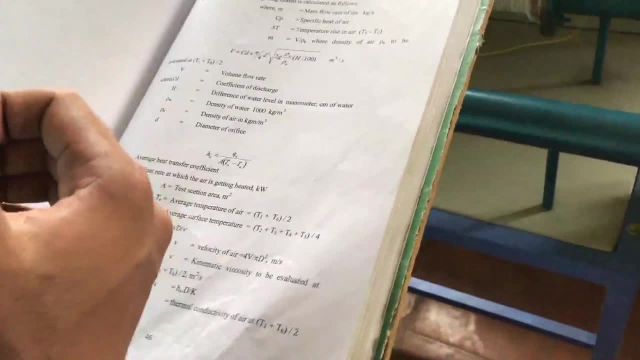 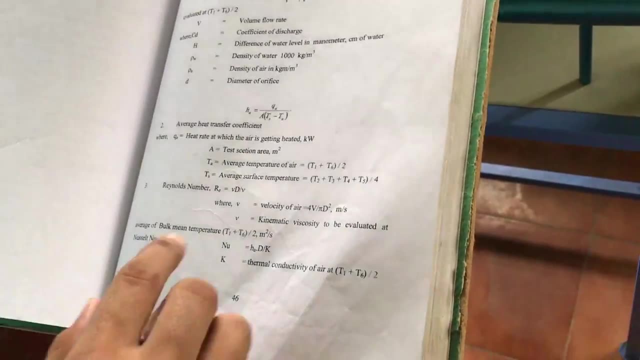 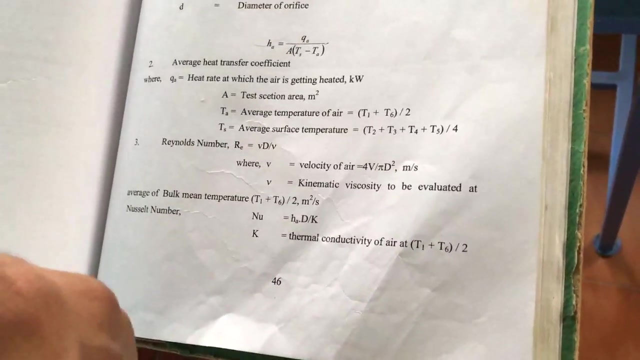 an average temperature. So from tables we are able to find the. this is an average kinematic viscosity of that particular temperature, and then we will be substituting that here, v, d by mu. here d is the diameter, diameter of the pipe is known, and v means v is the velocity of the velocity of. 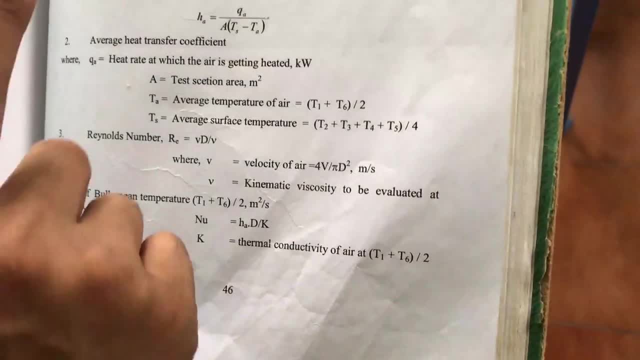 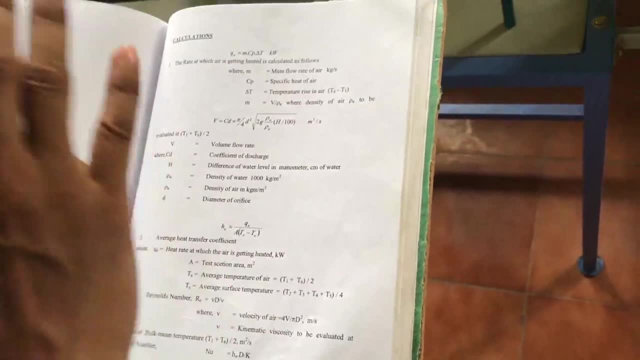 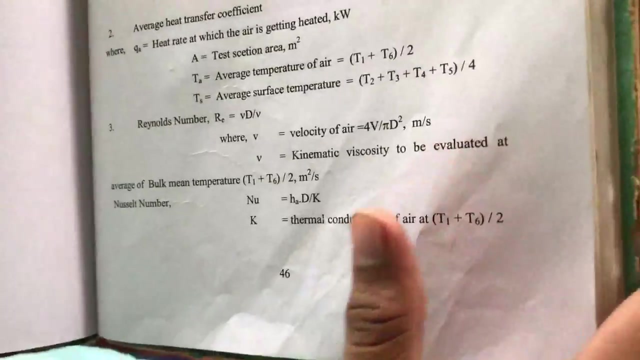 air for finding the velocity. what we do is we are having the volume, so that volume will be divided by the cross-sectional area. we will get the this one, we will get velocity, so that velocity will be substituted here and now. we are able to obtain so here, volume divided by cross-sectional area. 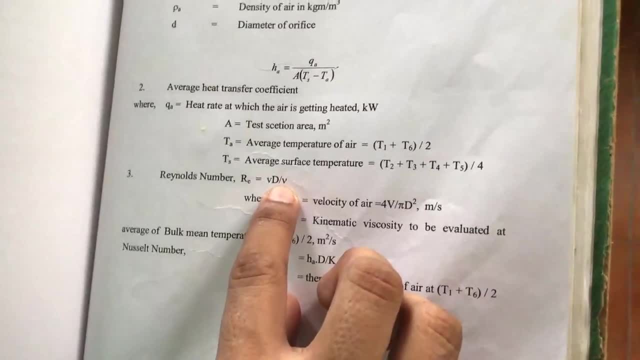 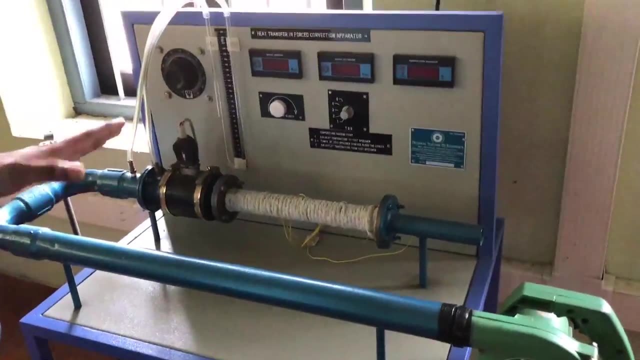 so we have velocity, this kinematic viscosity, and we will be substituting d and then we will get the Reynolds number. so this is how we find the getrenser coefficient and Reynolds number: by using using given apparatus. thank you you.